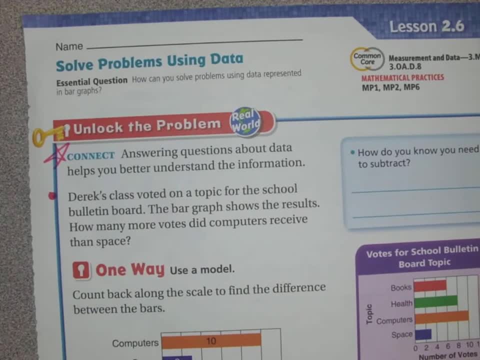 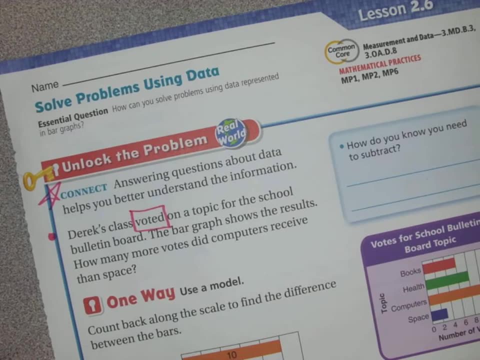 our word problem. Derek's class voted on a topic for the school bulletin board. Okay, so the class voted, So they're taking a survey, and the survey is in a bar graph. The bar graph shows the results. All right, so here's our. 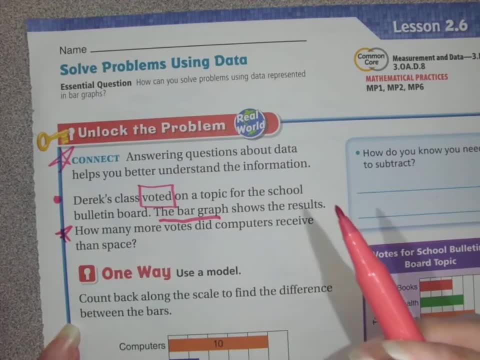 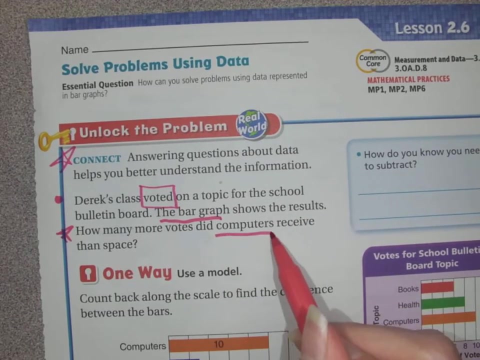 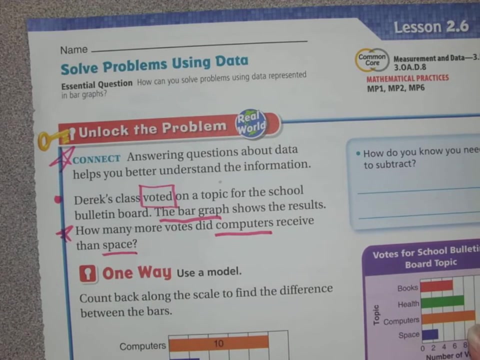 question: How many more? How many more votes did computers receive than space? All right, so we're comparing. We're comparing the number of computers, the number of votes computers received than space. So computers to space, that's what's being compared And we know the clue phrase: how many more means? 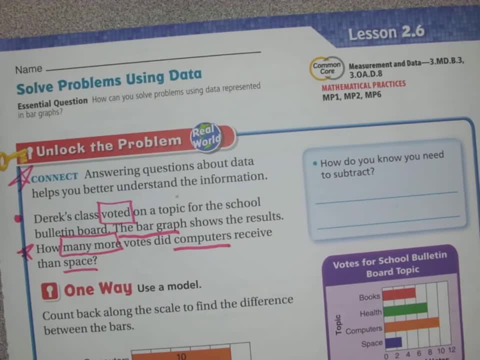 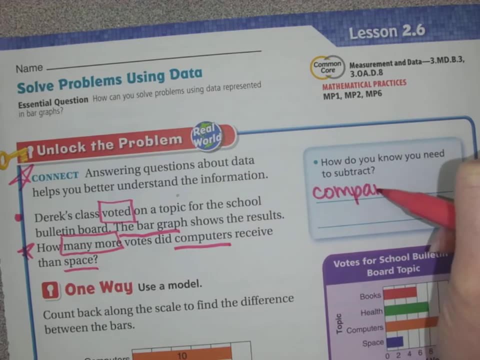 to subtract. Okay, and how do we know we need to subtract? Because we're comparing. we're comparing computer votes. I'm going to abbreviate Computer votes to space votes. That's how we know because of the question. All right, so let's look at one way, Let's use our model. Here is the. 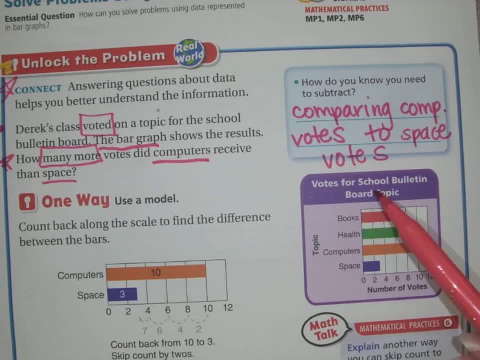 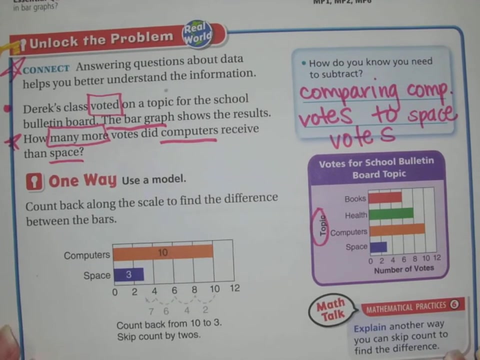 bar graph titled votes for school bulletin board. Here are all the topics: space, computers, health and books. Look at the bar. Here are the numbers that represent those topics And then down here the scale represents number of votes, from zero to 12. So we're skip counting by twos, All right, so one way we could count back. 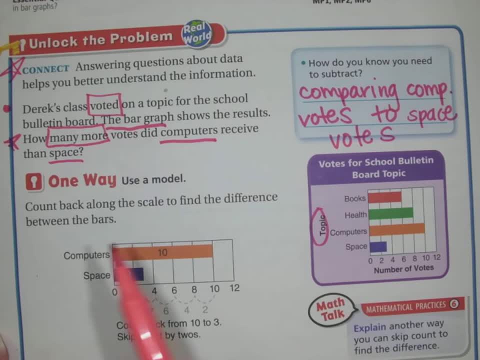 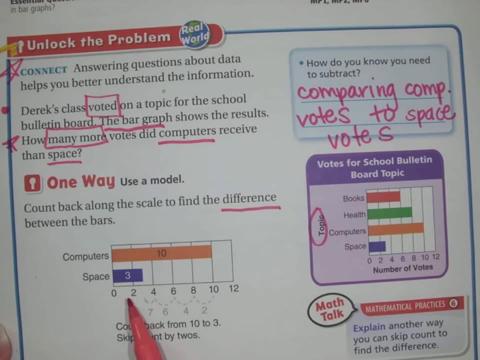 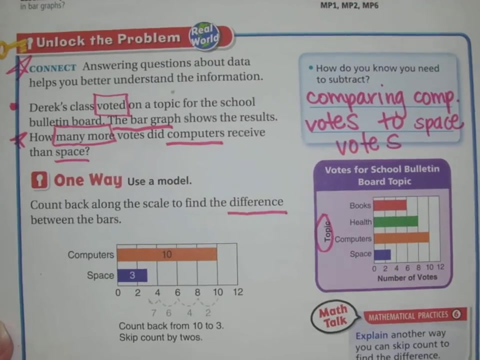 along the scale to find the difference between the bars. Okay, so we know. as you can see, computers definitely had more votes than space. Look at how long the bar is for computers and look how small space is. We need to know by how many more votes. So what they're showing you is to skip count. 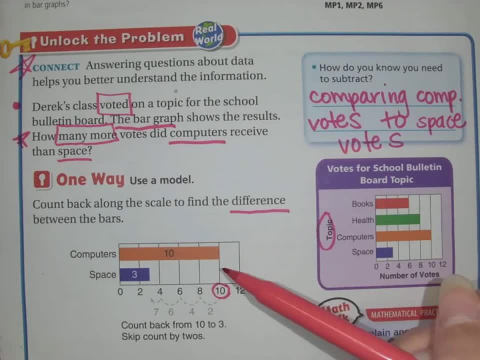 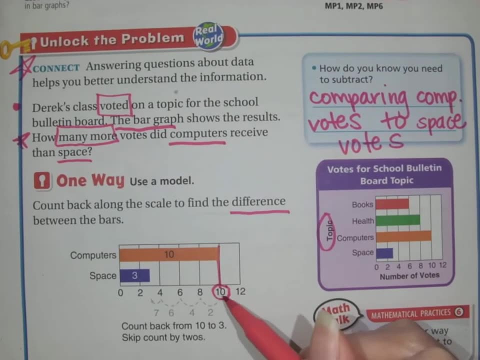 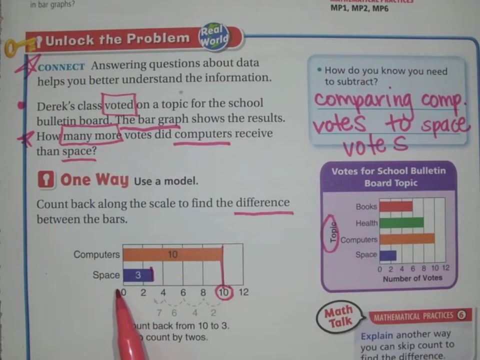 We would start at 10 right here, because computers had 10 votes and we would skip count back. skip, count by twos from 10 all the way to three, because three represents the number of votes space received, Right? So let's see: count back, start at 10, and count back by 2.. Because 3 represents the number of votes space received, right? So let's see: count back, start at 10, and count back by two. Okay, which was 10.. That's the second one. This is not the second one. 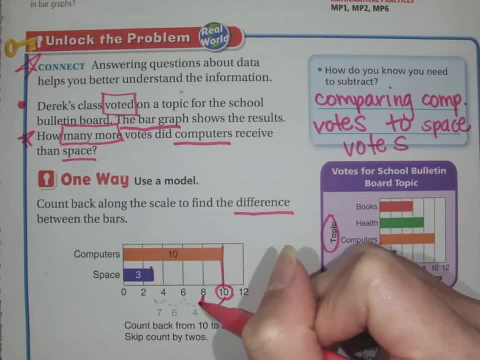 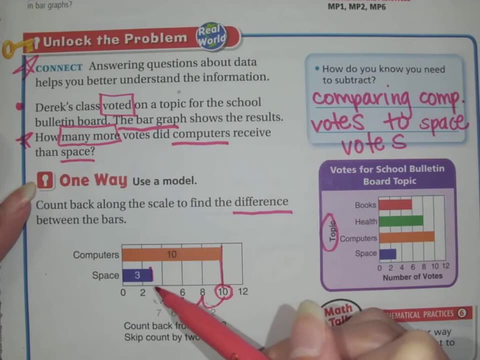 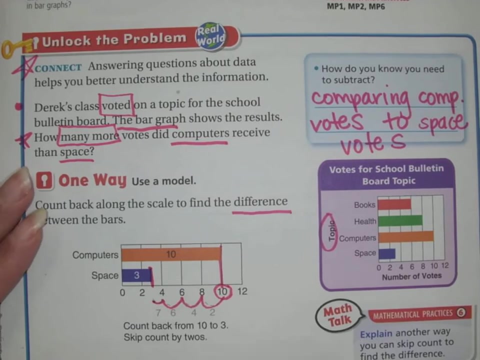 This is not the second one. This is not the second one. The third one is the third one. back by twos, Two, four, six, Instead of counting back to eight. remember this half of a bar. we would stop at seven, So the difference is seven votes. You can also just like we've been. 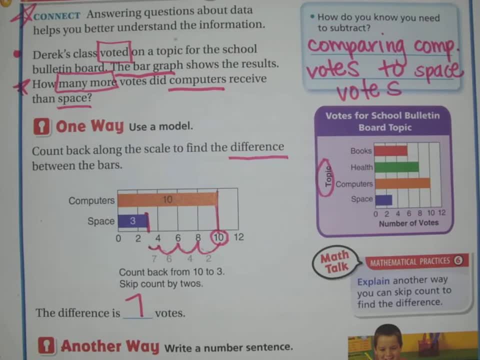 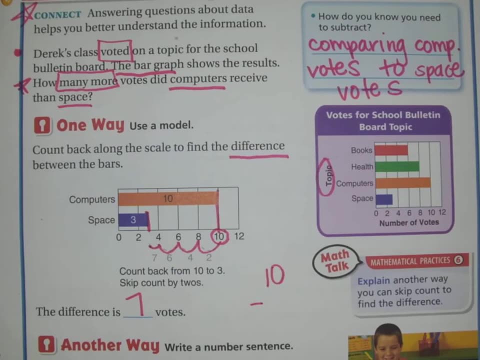 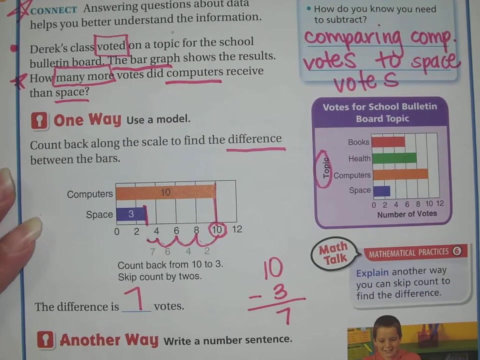 doing boys and girls. you can write a number sentence. We know again: computers received ten votes and we subtract the number of votes, space received, which was three and ten minus three, equals seven. I feel like a lot of you have been using that strategy, but whichever one you 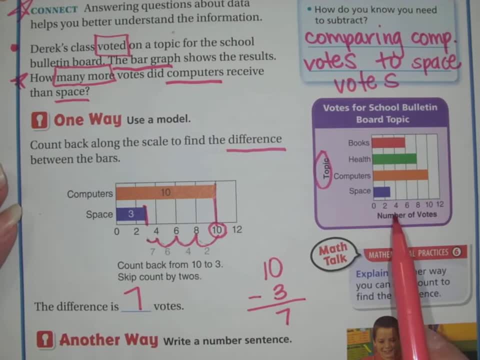 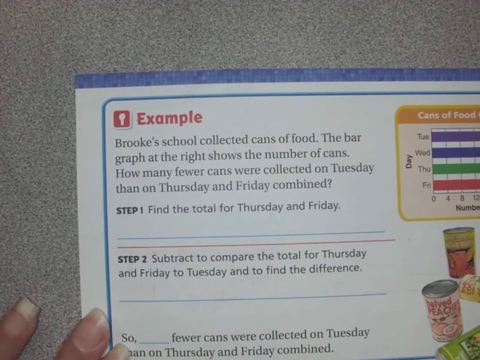 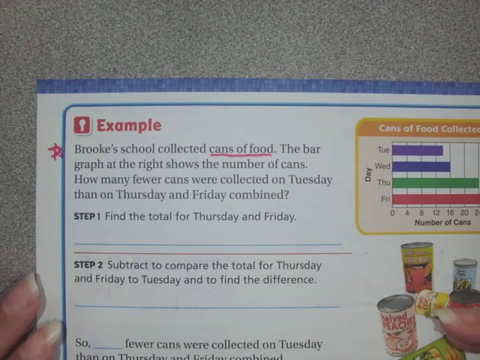 like You can count back on the scale. count back or you can subtract. Okay, so how many more votes do computers receive in space? Seven votes. Let's look at another one. Brooke's school collected cans of food- All right, cans of food. We're going to have a survey. 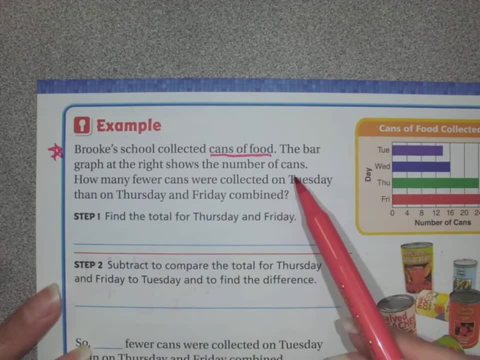 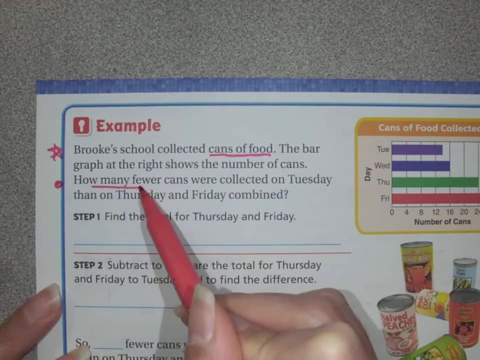 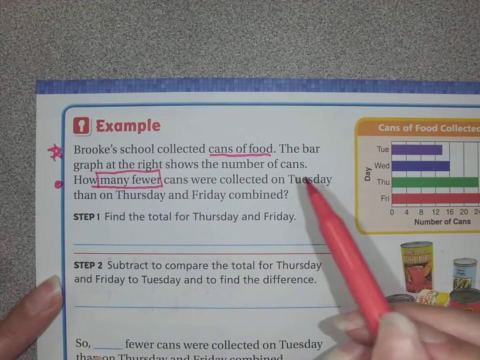 The bar graph at the right shows the number of cans. All right, here's the question, guys: How many fewer, how many fewer? oh, that means subtract, just like how many more, how many fewer cans were collected on Tuesday? 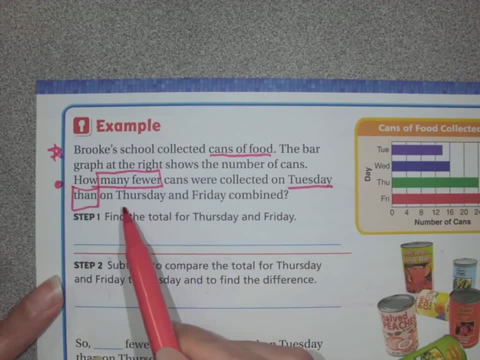 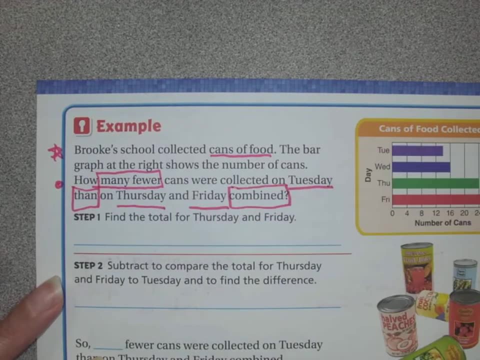 than- here's that clue word- than than on Thursday and Friday combined. Oh, okay, this, this is the sentence that has thrown some of our friends off. All right, we got this. So let's look In this question: how many fewer cans were collected on Tuesday? 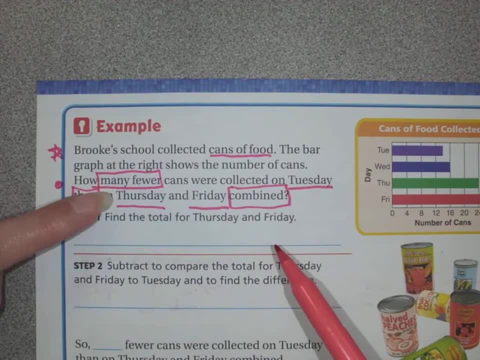 than on Thursday and Friday: combined, I see how many fewer. well, how many fewer means to subtract, and down here I see combined. I know combined means to find the total to add. So we're going to be doing two different things. 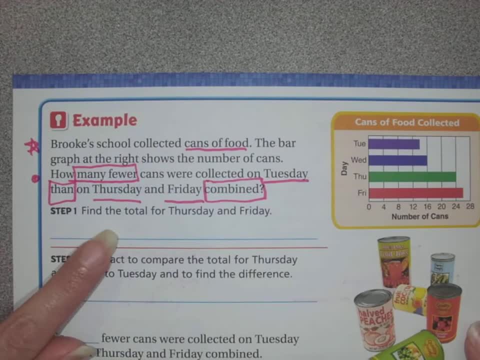 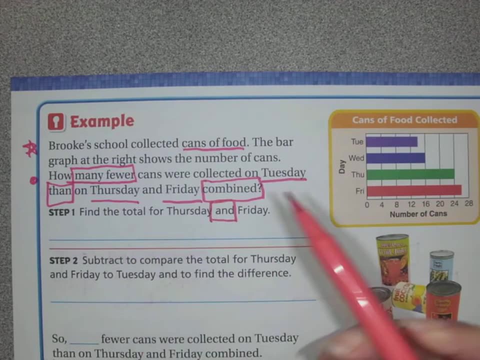 All right, step one: Let's first find the total for Thursday and Friday. Okay, remember, it said Thursday and Friday combined, So we're going to find these, the number of cans on the bar graph. So let's go and find Thursday first. boys and girls: Okay, 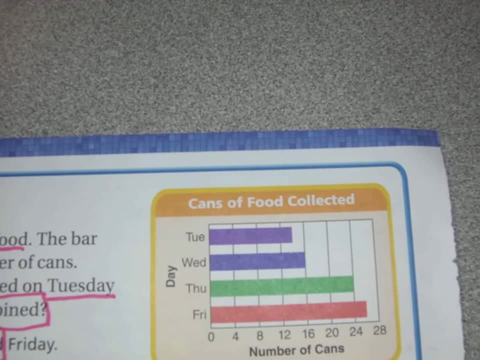 Make sure this all right. Thursday: here's the day of the week, right here. Here are the number of cans. So, Thursday: how many cans did they collect? Here's Thursday: starting from zero, go all the way down. 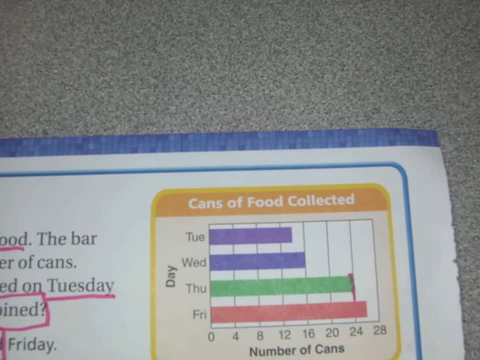 It ends right here. If I go down, that's at 24.. Okay, so I'm going to write 24 on my paper, And then Friday. how many cans did they collect on Friday? Here's Friday. Now I'm going to go all the way down. 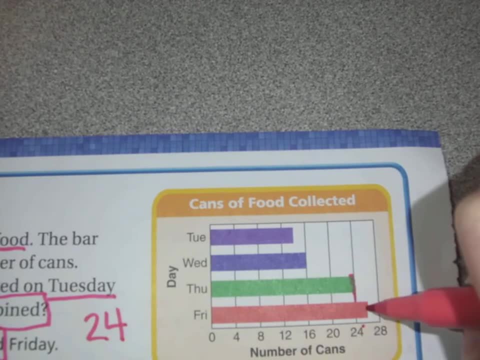 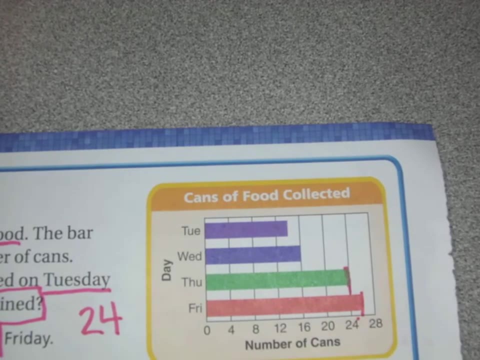 Okay, so I'm going to go all the way down Until the bar ends. and it's right here. All right, I got to think a little bit on this one. Okay, so it's in between 24 and 28.. Well, you have to think, boys and girls. 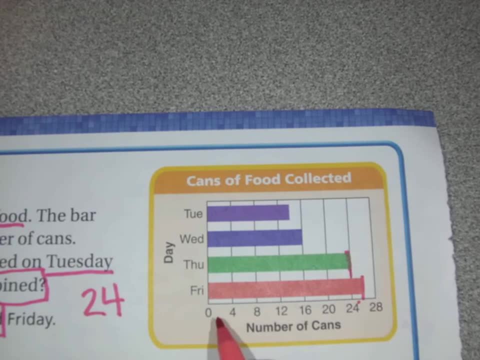 Look at the scale. The scale is from zero. So, from here to this line, that represents four cans. From here to here. So we're skip counting by fours, right? So let's think. So we're skip counting by fours, What would go in between 24,, 25,, 26, or 27?? 24,, 25,, 26,, 27.. 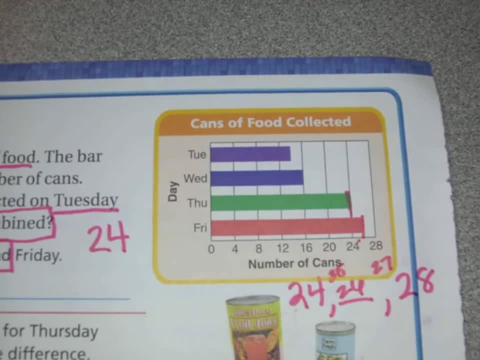 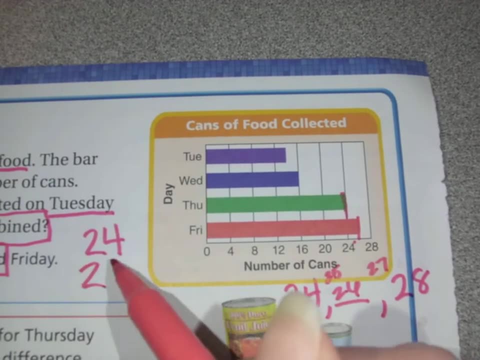 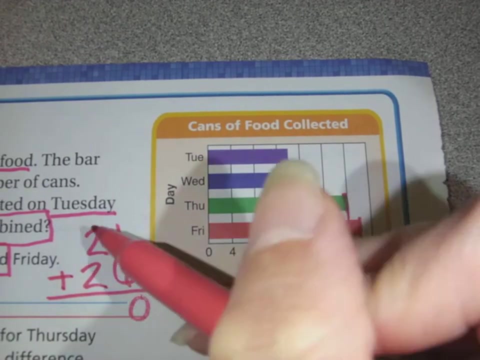 So what's in between 25 and 27?? Oops, 26.. Okay, so they collected 26 cans on Friday, All right, so we need to add these up first. 26 plus 4 ones is 10 ones. Regroup. 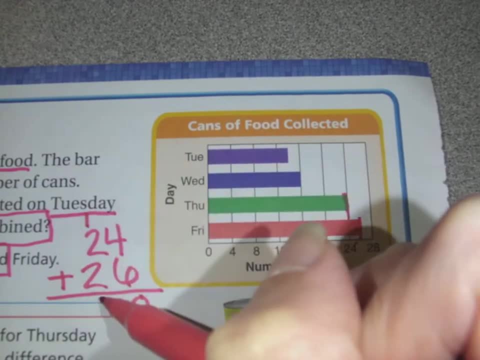 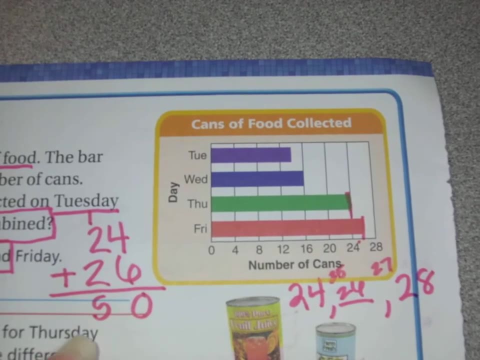 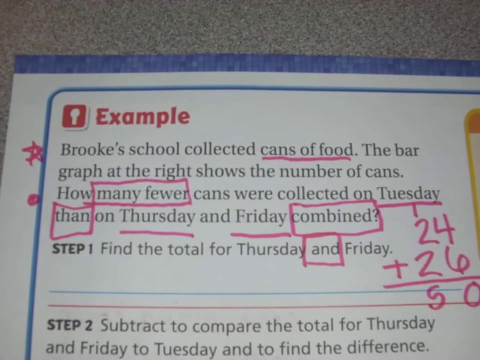 2 plus 2 tens is 4 tens plus 1 is 5 tens. So Thursday and Friday combined, the total number is 50.. Okay, we're not done yet. Let's come back to this question. It said how many fewer cans were collected on Tuesday than on Thursday and Friday combined. 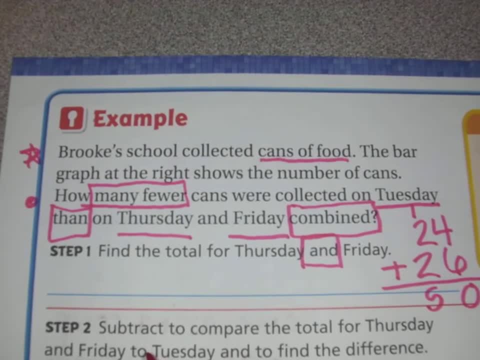 So we already combined Thursday and Friday. So now we're going to subtract, to compare the total For Thursday and Friday to Tuesday and find the difference All right. so let's see how many cans were collected on Tuesday because, as you can see, Tuesday got. 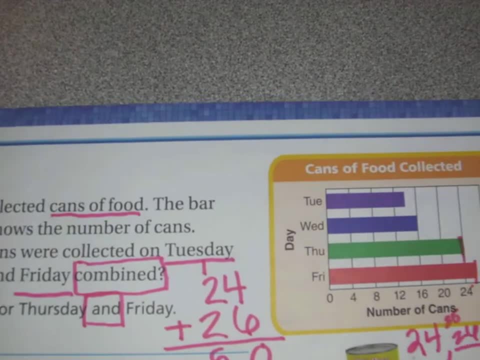 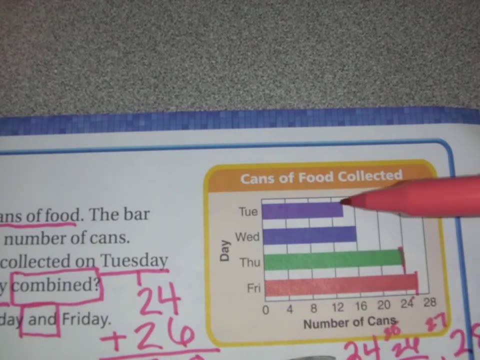 They had the fewest amount of cans that were collected. Sorry about that. So let's look at Tuesday. Here's Tuesday. Go all the way down. Well, this is where it ends, Right here, It's in the middle. Let me go down. 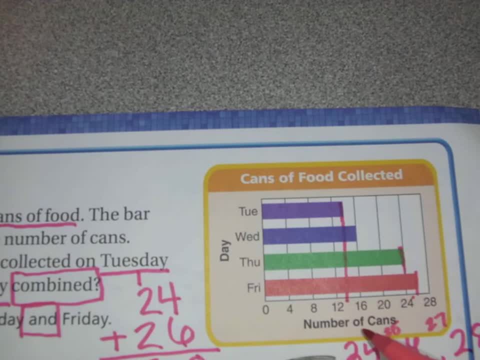 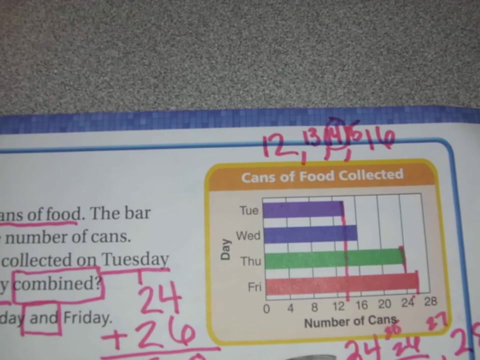 All right, so it's in between 12 and 16.. 12 and 16, 13,, 14,, 15, so look here, 14 is in the middle. So 14 cans were collected on Tuesday, So we're going to take 14. 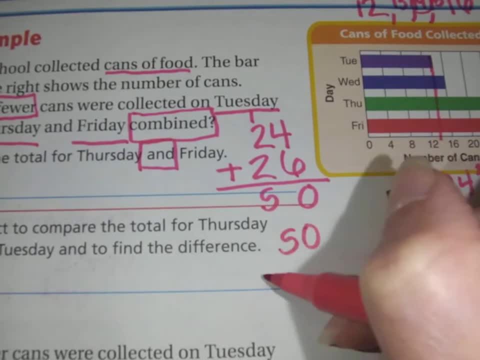 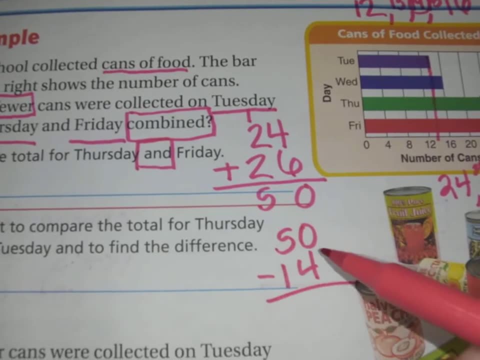 and we're going to subtract it from 50.. 50 minus 14.. Okay, Let's subtract. We have to regroup, We do not have enough. not have enough to take four from zero. Take a ten. That one ten becomes ten ones, Ten plus zero. 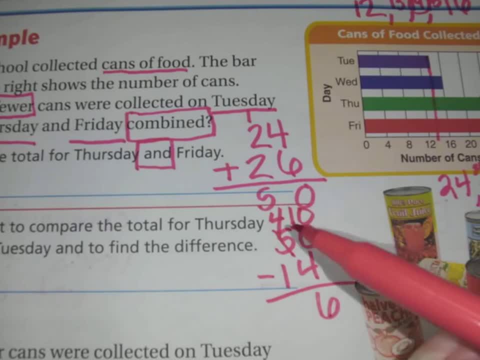 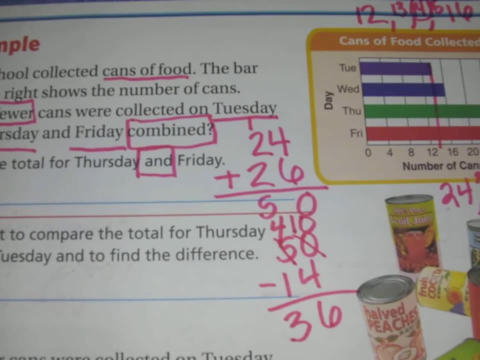 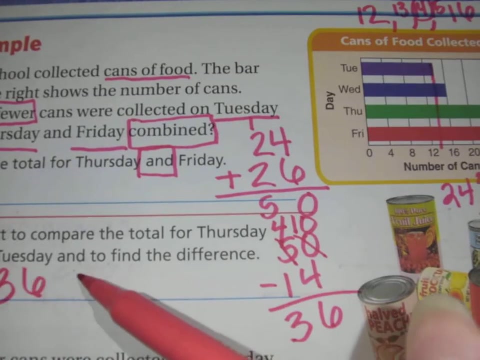 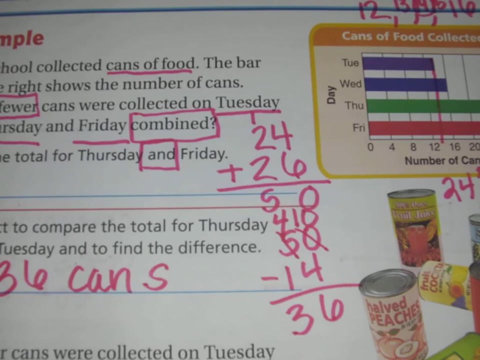 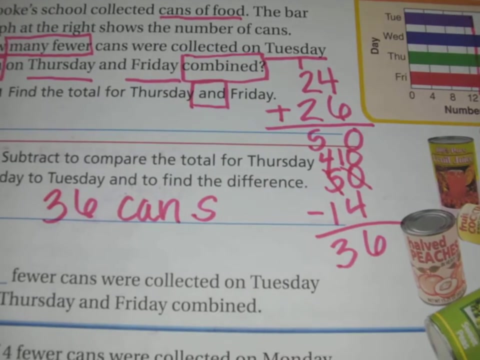 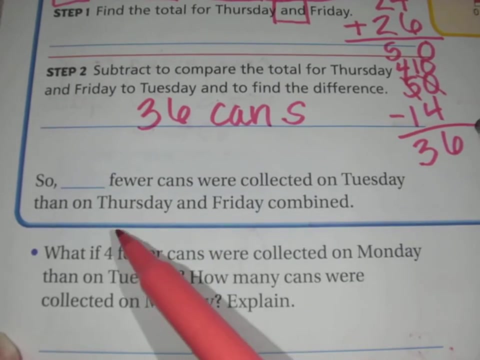 is ten. Ten minus four is six. Four minus one is three: Thirty-six. So how many fewer cans were collected on Tuesday than on Thursday and Friday combined? Thirty-six cans, All right, let's look at. let's do another one. All right, let's look at this one. right here. It says: what if four? 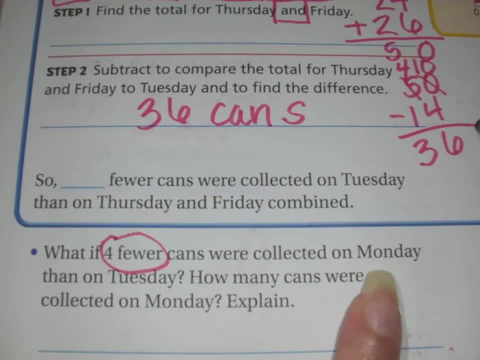 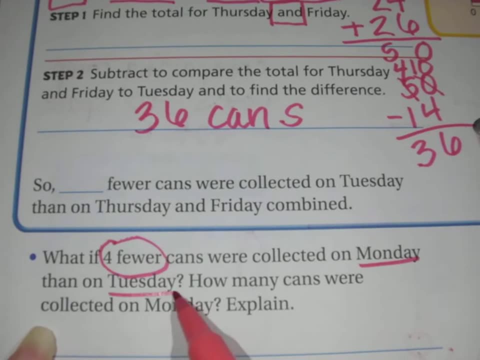 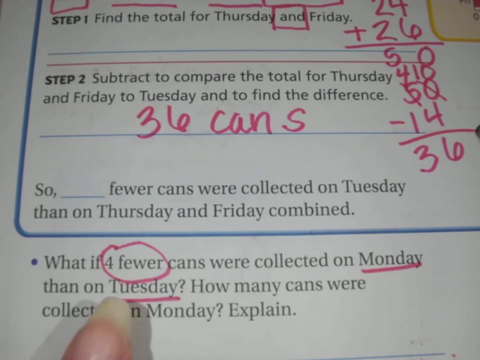 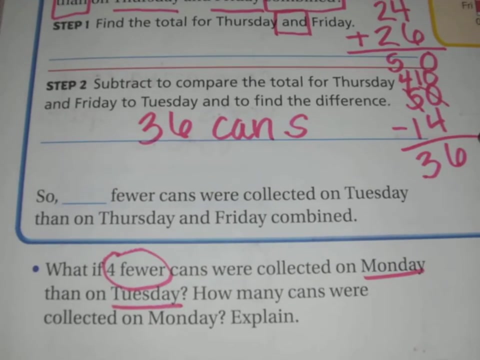 fewer cans were collected. How many cans were collected on Monday than on Tuesday? Okay, so we're comparing Monday to Tuesday. How many cans were collected on Monday? All right, so four, think four fewer means less. What if four fewer cans were collected on Monday than on Tuesday? All right, so let's see. 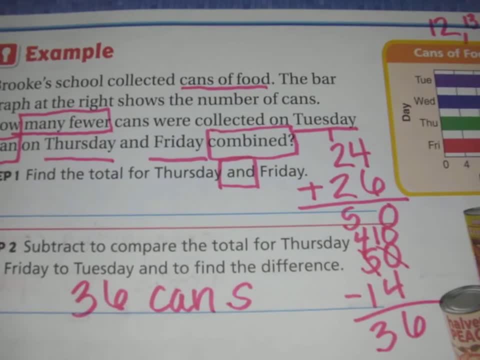 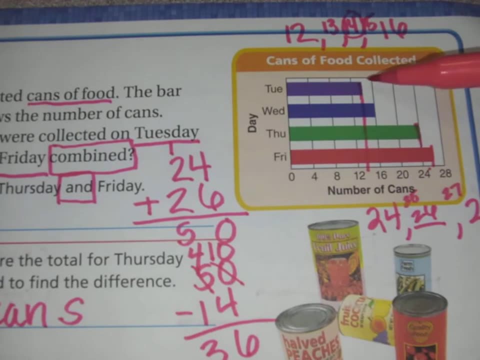 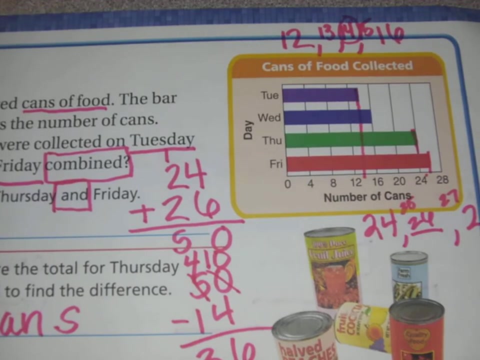 How many cans were collected on Tuesday? again, Because we need Tuesday's information. Tuesday up here we said 24.. And what if four fewer cans were collected on Monday than on Tuesday? 24 minus four. I'm sorry guys, I'm sorry, I made a mistake. I don't know why I said 24.. 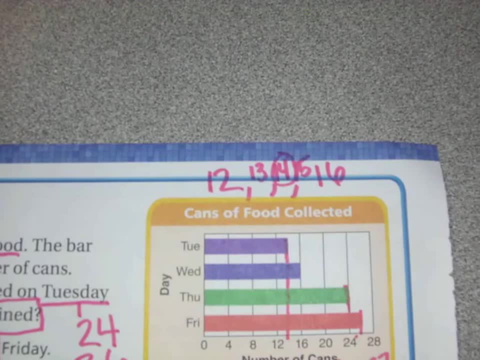 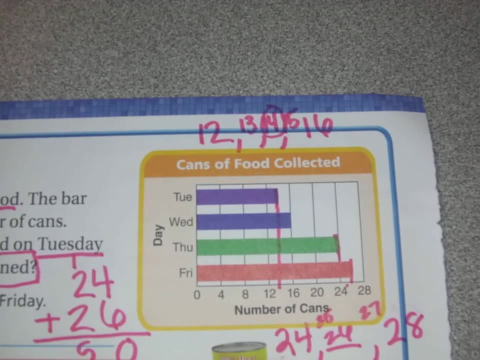 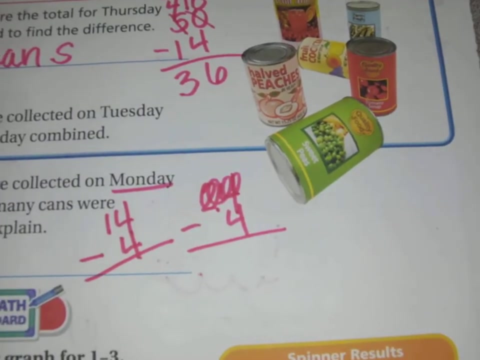 Let's look at Tuesday's number of cans 14.. Excuse me, guys, 14 represents the number of cans that were collected on Tuesday. So 14 minus four, And 14 minus four equals 10.. So how many cans were collected on Monday? 10 cans. 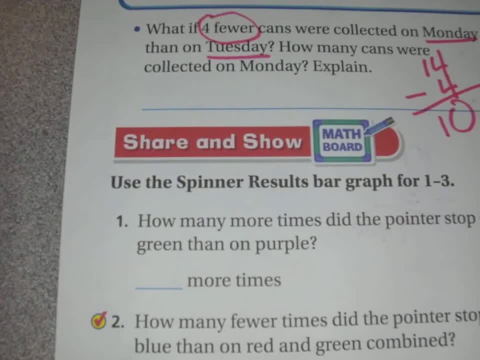 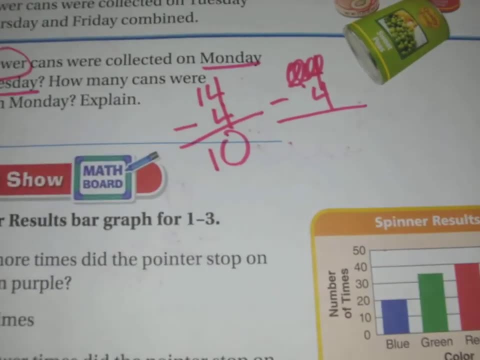 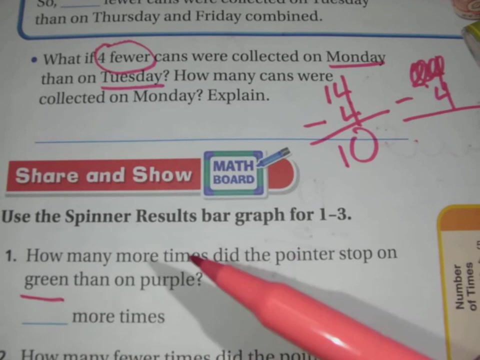 All right, we'll do one more. Let's look at the spinner results. The spinner results, All right. It says the question says: how many more times did the pointer stop on green than on purple? So we're comparing green, the color, green to the color. 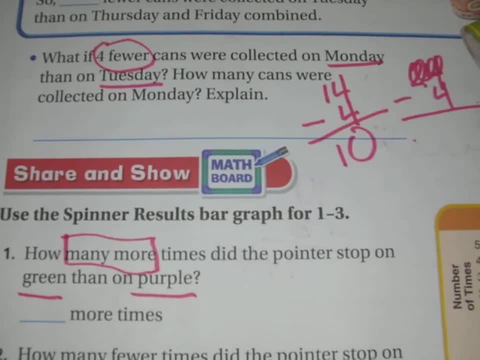 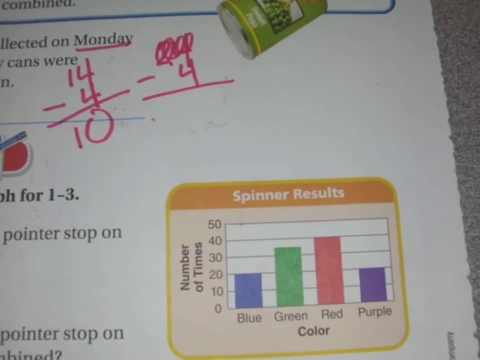 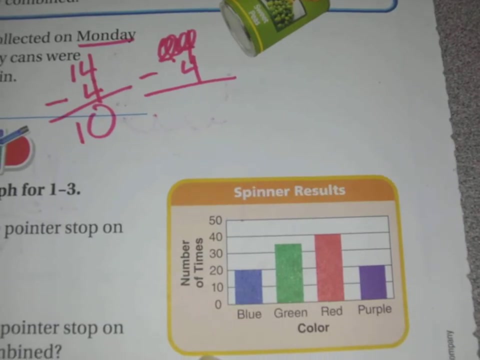 purple. And we know how many more means to subtract. So let's see how number of times green was spun. All right, Well, let's look here. Our scale is 14. And we know how many more is from zero to 50. So it's counting by tens. All right, green, Let's see Number. green, Let's. 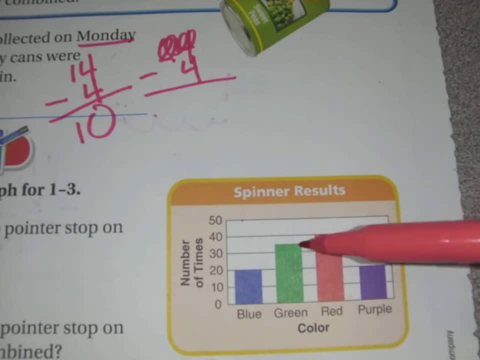 start right here. The color green go up, Stops right here And you got to think what's in between 30 and 40. That's 35. And let's find purple- Purple's right here And it stops right here And 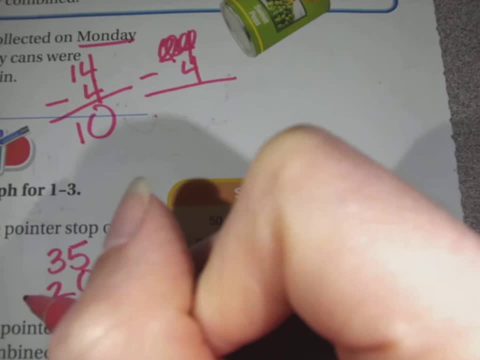 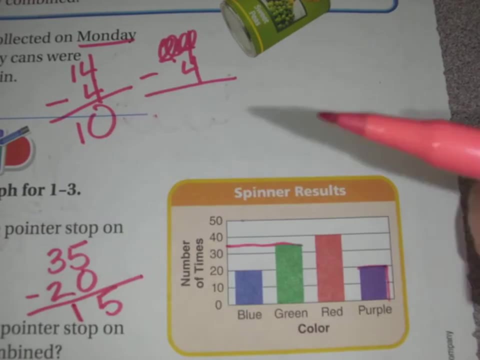 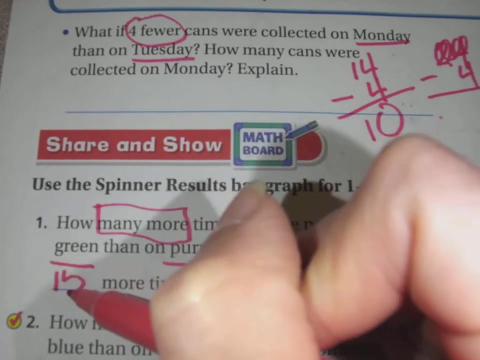 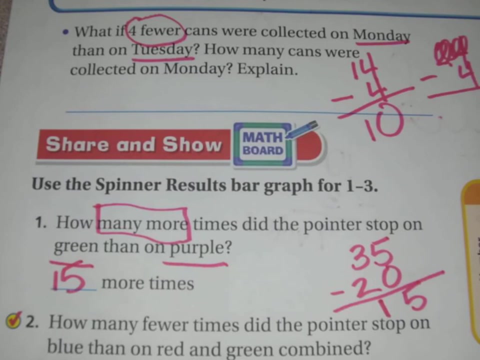 that is exactly at 20.. So we can subtract: Five minus zero is five, Three minus two is one. So how many more times did the pointer stop on green than on purple? 15 more times, And that was basically you guys. some practice on how to solve problems using data represented on bar graphs.